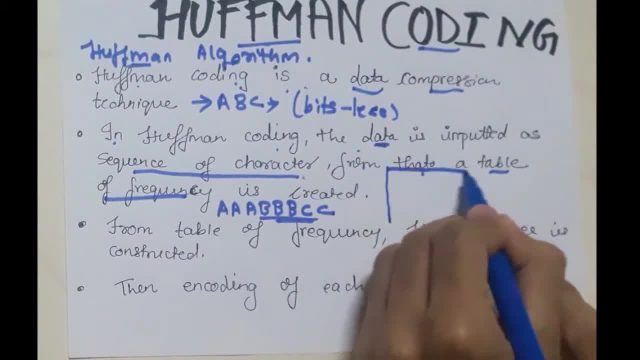 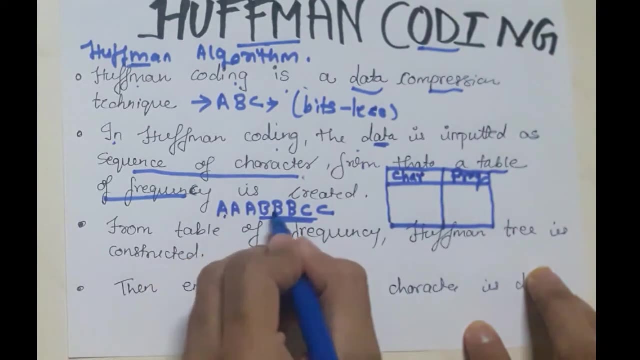 table of frequency is created. see Your character and your frequency. See, in this sequence you can see there are three types of characters: A, B and C. right, So we will write here: A, B and C. So these three characters are there in this sequence. Now frequency Now. 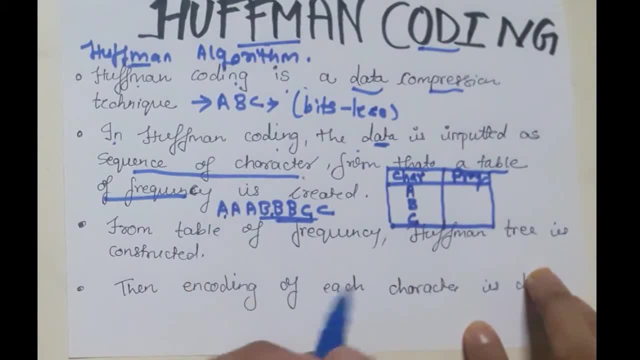 frequency, How we will calculate frequency. So frequency is dependent upon the number of times that character has occurred in the sequence. So occurrence of character in the sequence On that the frequency is dependent. See here: in this sequence A has occurred. 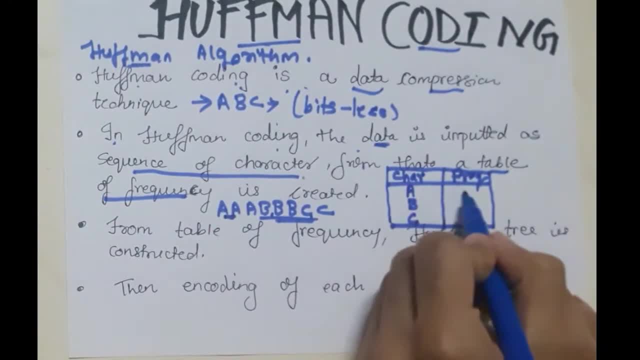 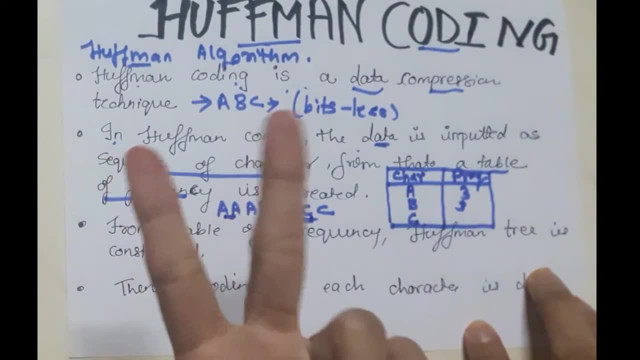 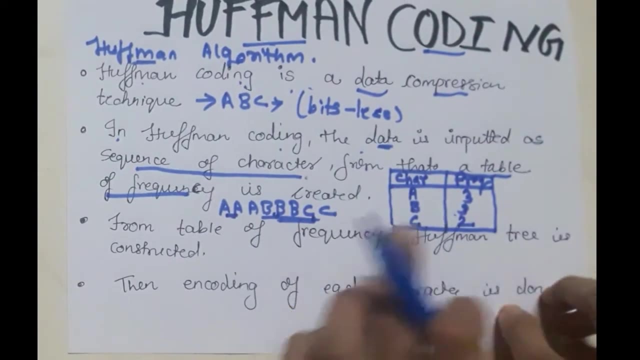 three times, right. So frequency of A is three. B has occurred three times in this sequence, So frequency is three, And C has occurred two times, So frequency is two. Now, like this, a table of frequency is created. From table of frequency, Huffman tree is constructed. 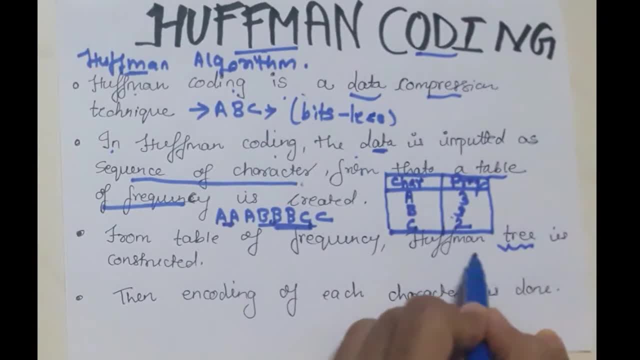 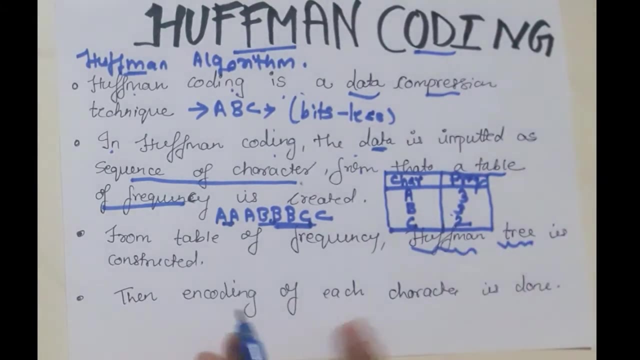 So, from this tree, what we will construct, We will construct Huffman tree. okay, From this table, from table of frequency, Huffman tree is constructed. okay, Then encoding of each character is done. And then, after construction of Huffman tree is done, encoding. 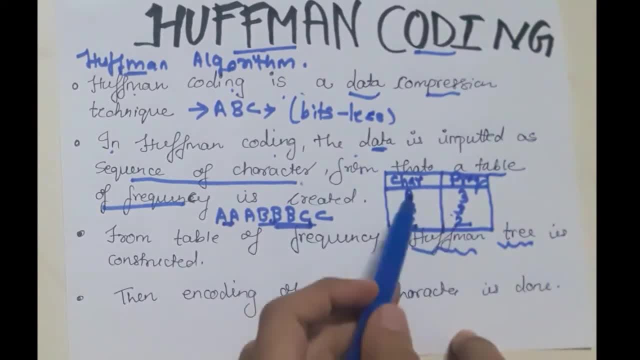 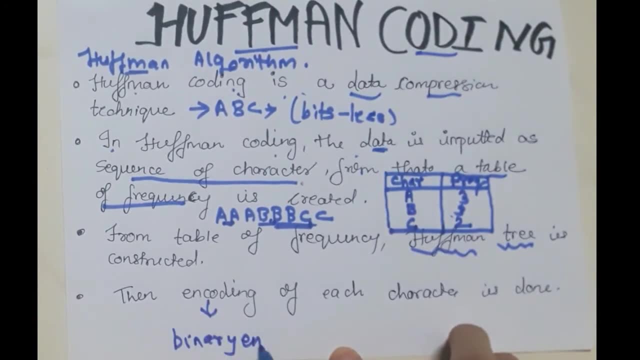 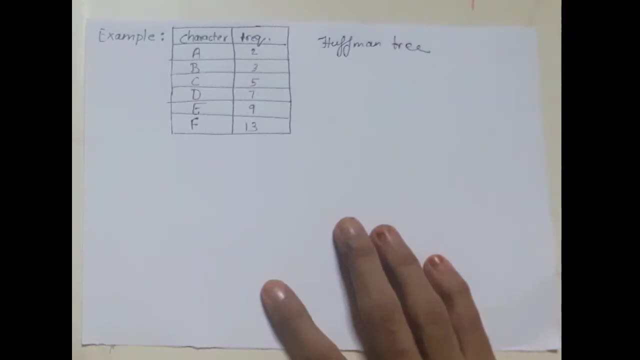 of each character is done. Here there are three types of characters, So encoding of all these three characters will be done And that encoding will be binary encoding. Okay, Now consider this example. So a table of frequency is given to you And you have. 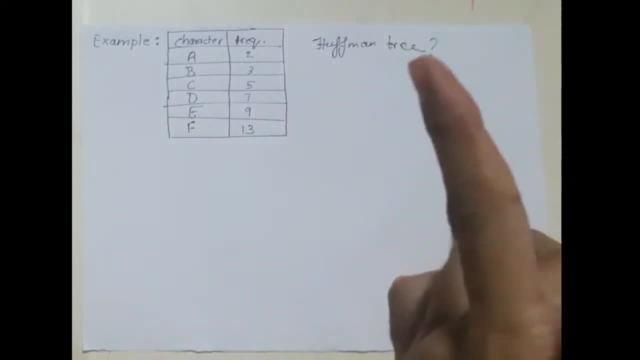 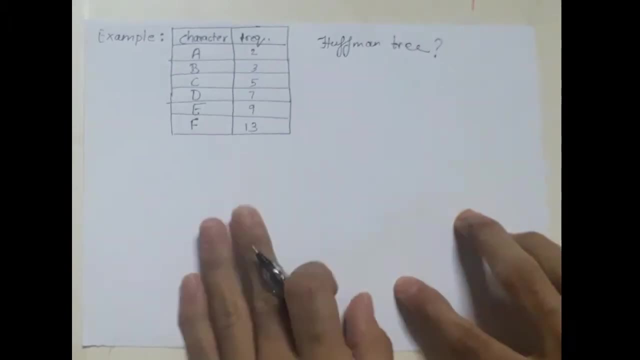 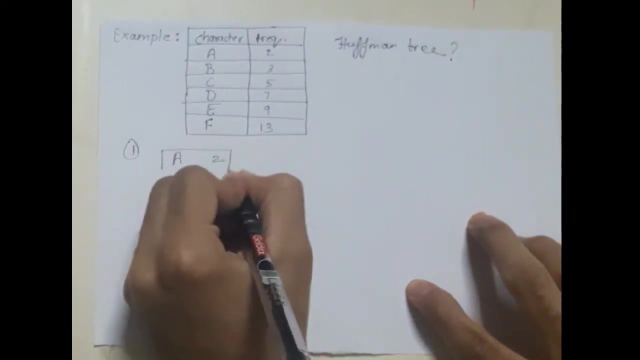 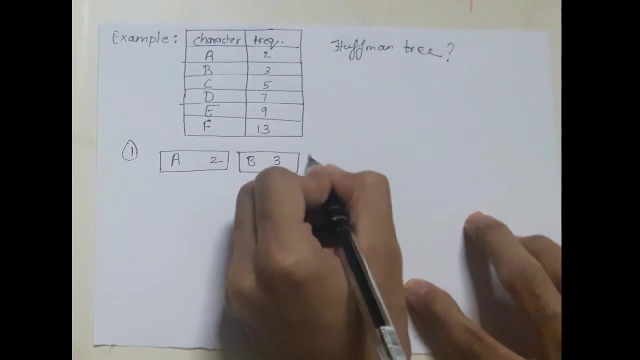 to construct Huffman tree from this table. Okay So, in first step, what we will do, We will arrange these characters in increasing order of their frequencies. Okay So, step one: C, frequency 2, C, frequency 10.. Like this, we will arrange these characters in increasing order of their frequencies. 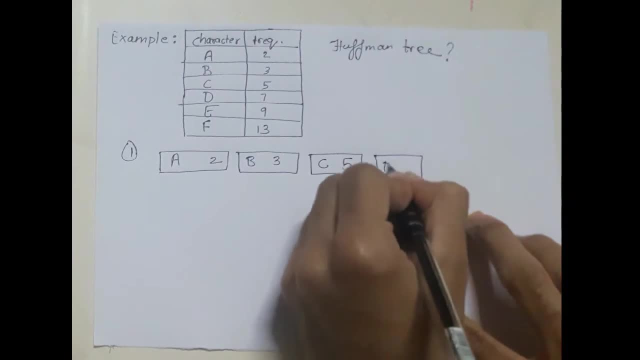 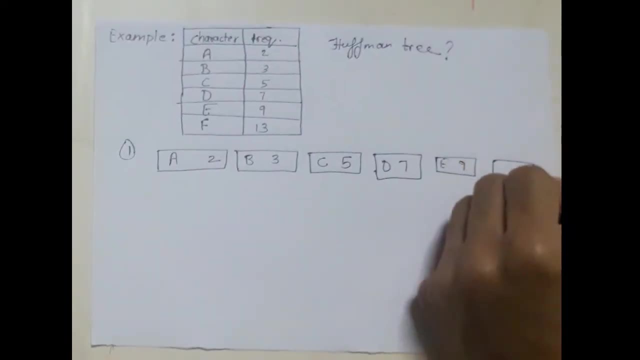 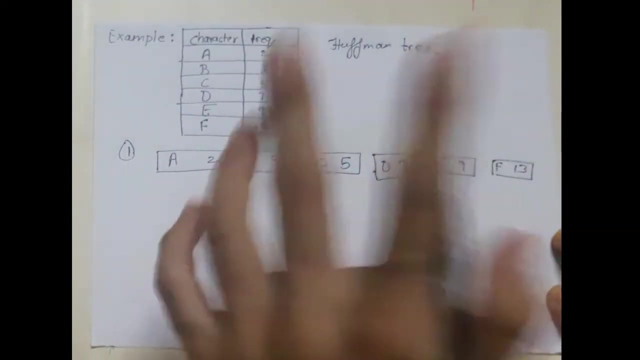 Okay, C- frequency 5, D with frequency 7, E with frequency 9 and F with frequency 30. Okay, Like this we have to arrange other. Now the next step is to select two, two characters from this which have least frequency. 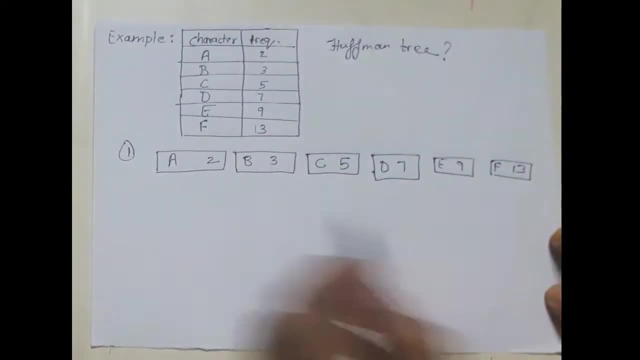 Among these all, we have to select two characters which have least frequencies. So those are A and B. See: A has 2 and B has 3.. So these two have least frequency among all. right, So we'll take these two. 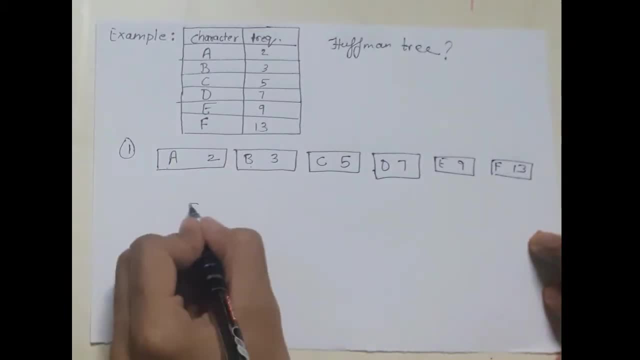 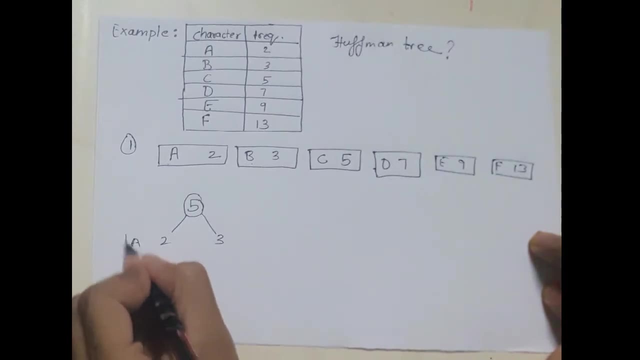 What we'll do. We'll merge these two, We'll merge 2 and 3 and we'll create a parent node like this: 2 plus 3 is 5, right. So now 5 is the parent of these two, right. 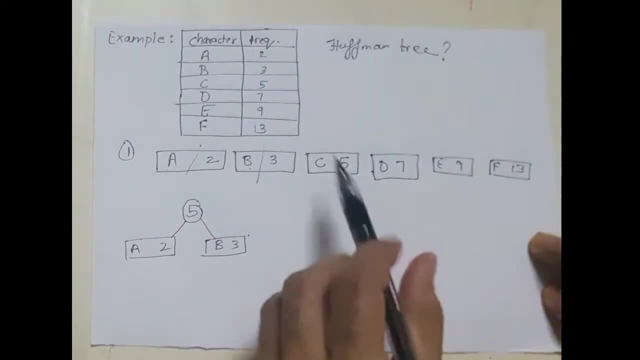 So we'll cut these two because we are done with it Remaining, we'll put. we'll take it down like this: C5, D7, E9, F13, okay, Now, from this 5, we have to cut this 2.. 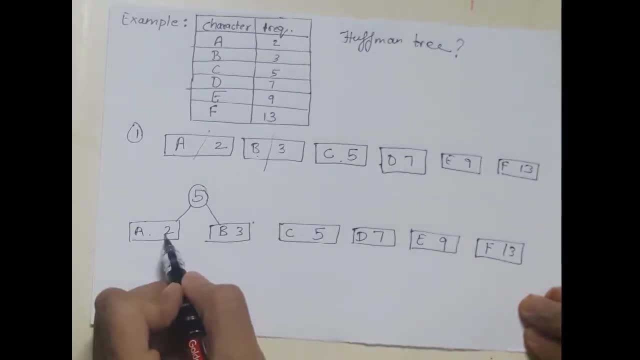 We have to select Now. we'll not consider this 2 and 3, huh, We'll consider this 5.. 5, then C5, D7,, E9 and F13, okay, So out of this 5, we have to take two characters which have least frequency. 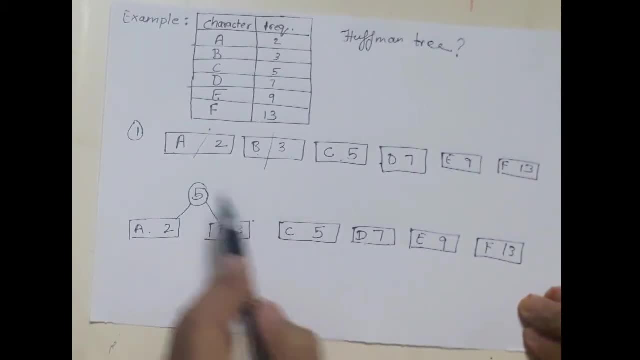 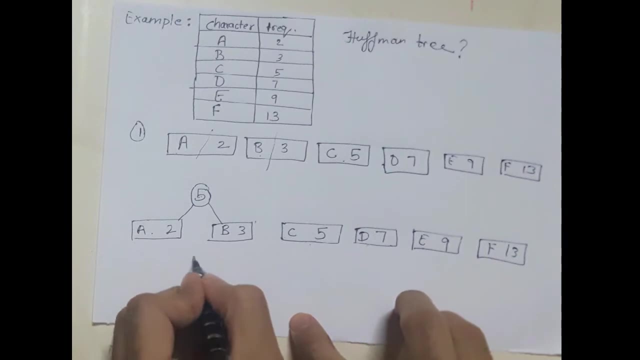 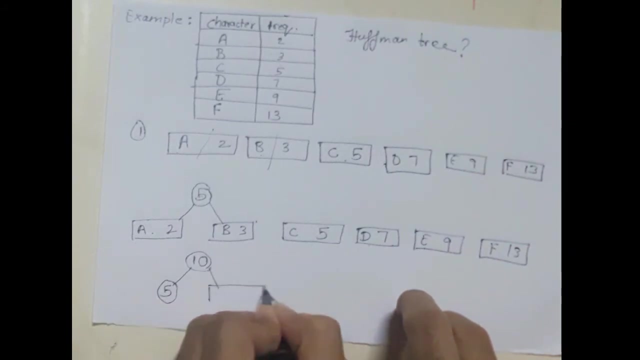 So here you can see this 5 and this. These two have least frequency. So again, what we'll do? We'll merge both of them. So 5 plus 5 is 10.. So 10 will get here 5, C5, this 5 is formed by A and B, A2, B3, okay. 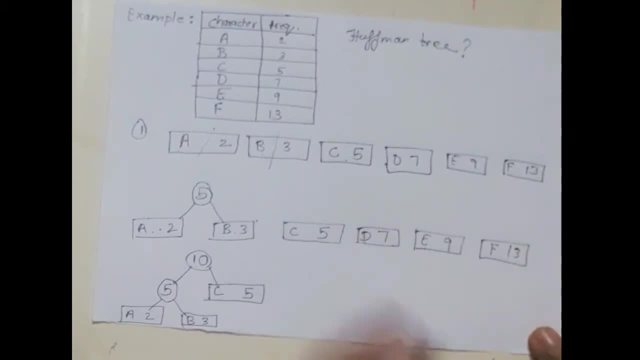 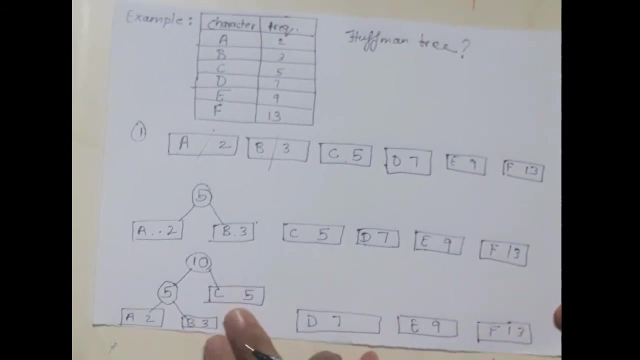 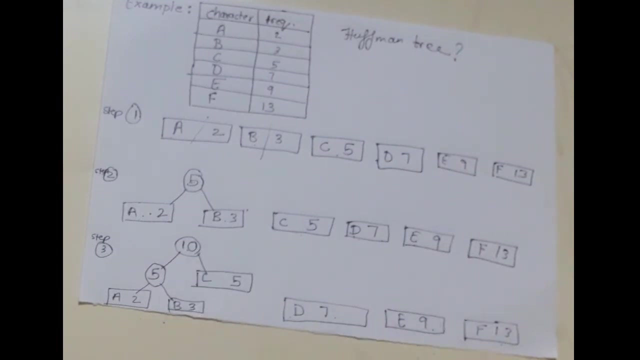 Now again, we'll take this down. this remaining 3, D, E and F- we'll take it down. okay. D7, E9.. F13, okay, Like this. Now again, out of this 4, we have to select two characters with least frequency. 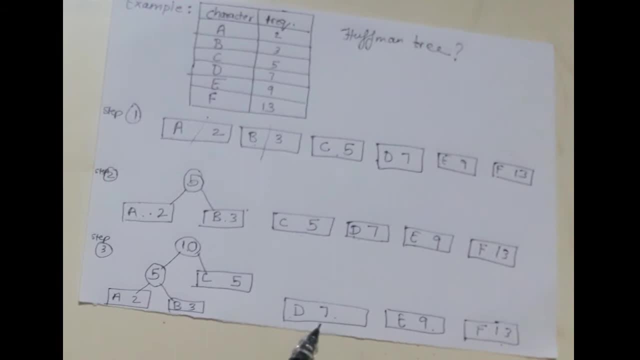 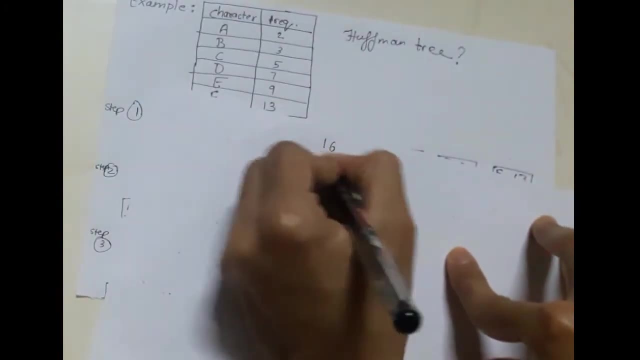 So here D and E have least frequency, So we'll merge these two. So 7 plus 9 is 16.. So we'll get 16 as the parent node, okay, So here I'll write 16.. And it is formed by B7 and. 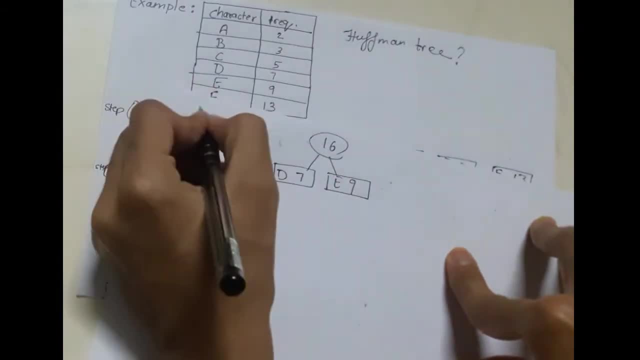 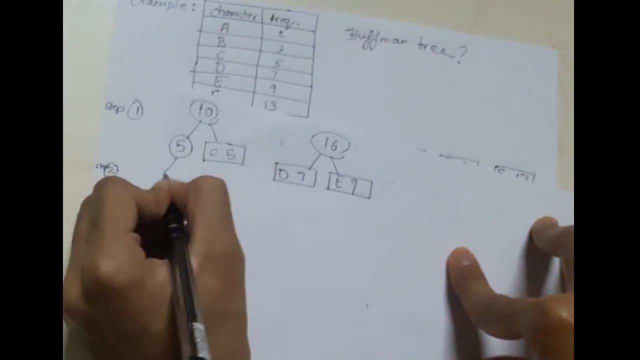 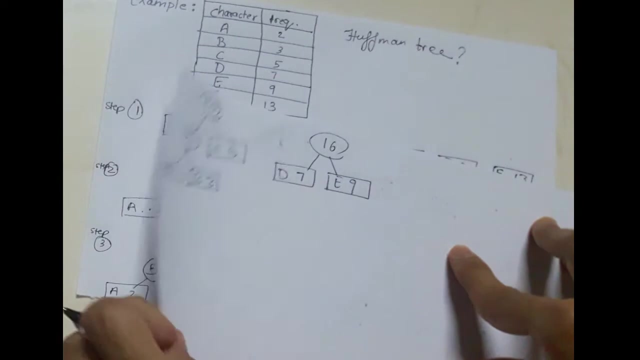 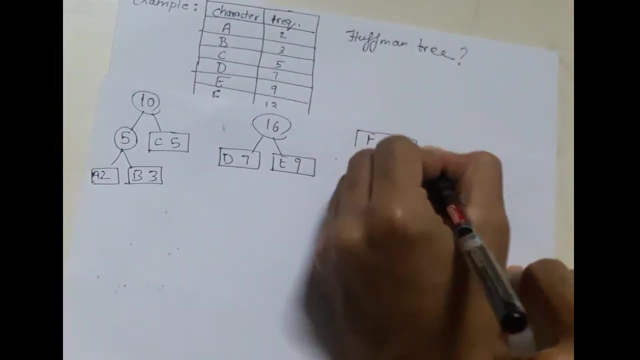 E9,. okay, And this 10 will be as it is. So 10, it is formed by 5. And here, F13, it will be as it is, okay. Now again, out of this 3, we have to select two characters with least frequency. 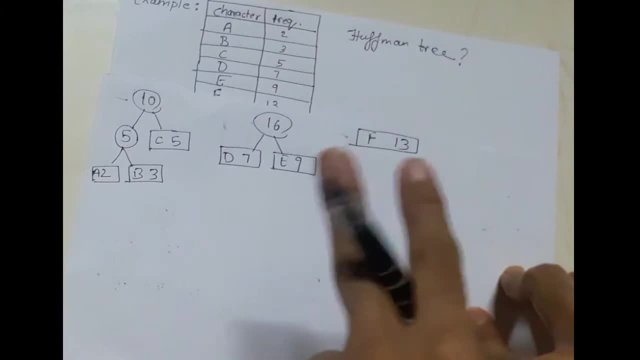 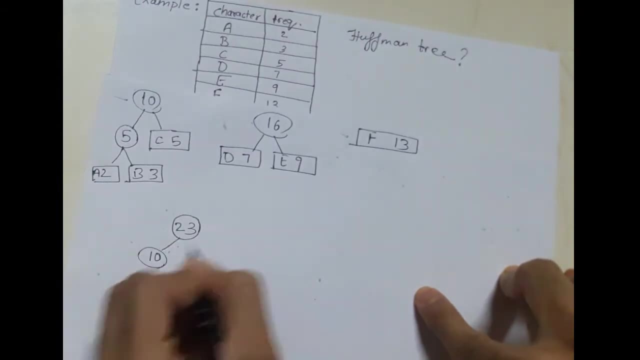 So 10 and 13 have the least, So we'll merge them. So 10 plus 13 is 23,. okay, So here, 23,, 10.. And this will be as it is, this sub-tree, okay, Okay. 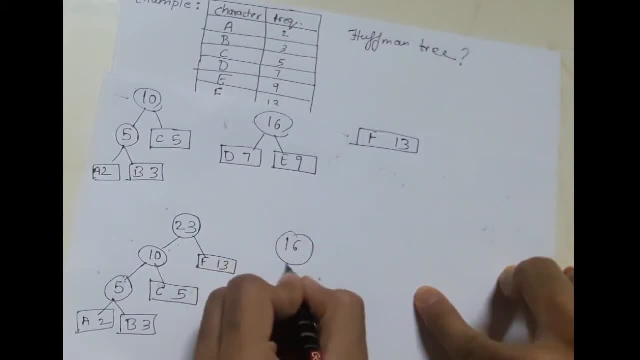 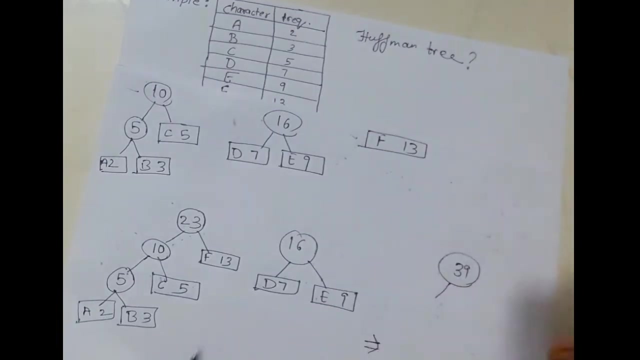 And this 16.. So we'll merge these two, because only two are remaining. okay, So we'll merge these two. So 23 and 16 together 39.. Okay, So this will be our final half-man tree. Now, always remember: out of these two, 16 has minimum frequency. 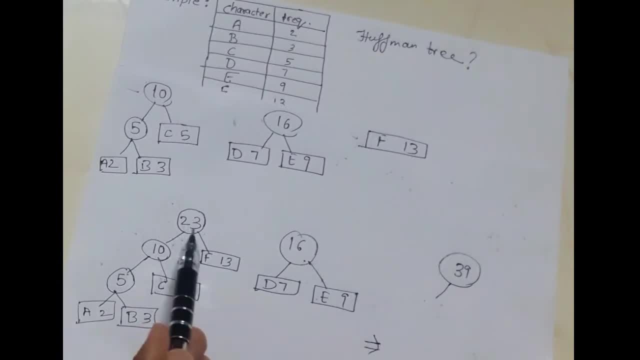 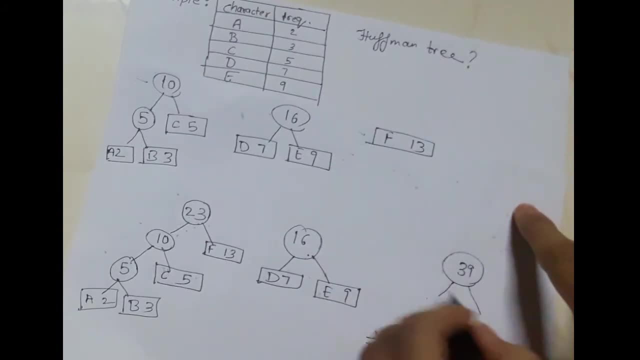 So the character with minimum frequency will be on the left-hand side And the character with greater than this will be on the right-hand side. okay Here, 16 has minimum frequency, So it will be on the left, And 23 has greater frequency. 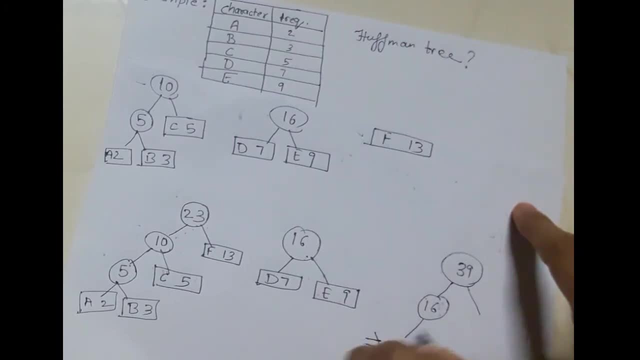 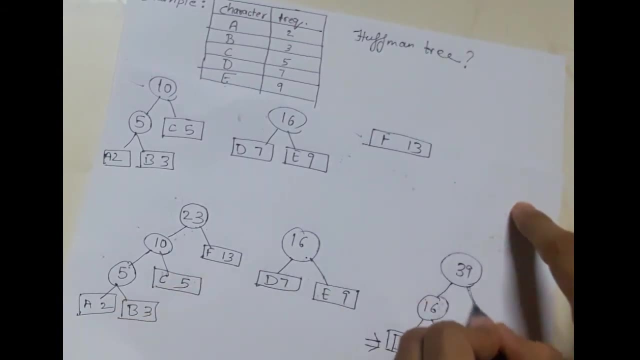 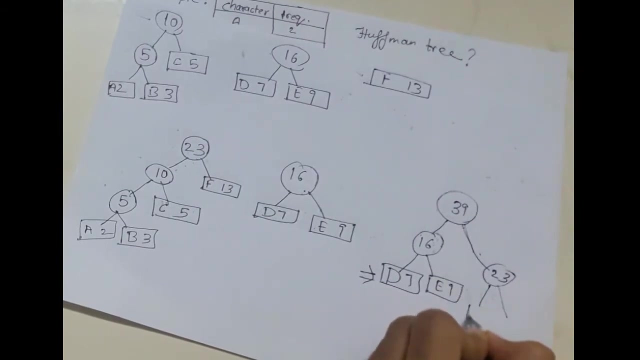 So it will be on the right. okay, 16 as it is: B7., E9., 23. E4., E5., E6., E7., E6., E7., E7., E8., E9.. 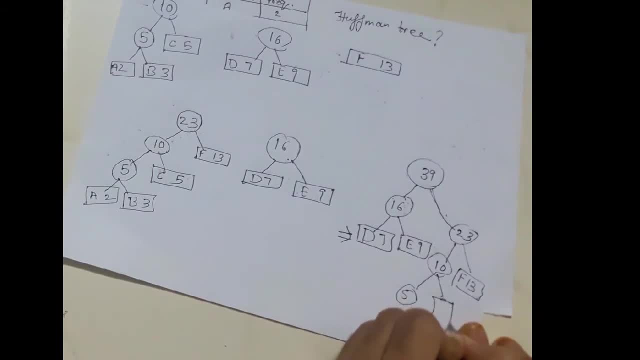 E9., E8., E9., E9., E9., E10., E11., E11., E12., E13., E13., E14., E15., E15., E16., E16., E17.. 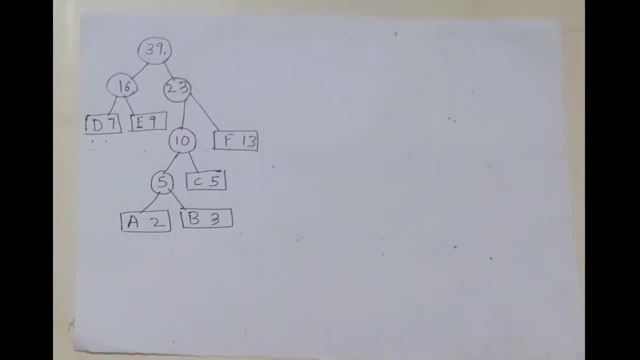 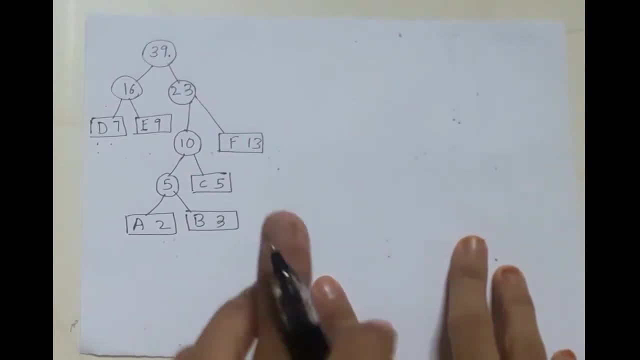 E18., E19., E19., E20., E21.. Now the next step is to assign 0 and 1 to this half-man tree. Okay, so 0 will be assigned on the left side and 1 will be assigned on the right side. 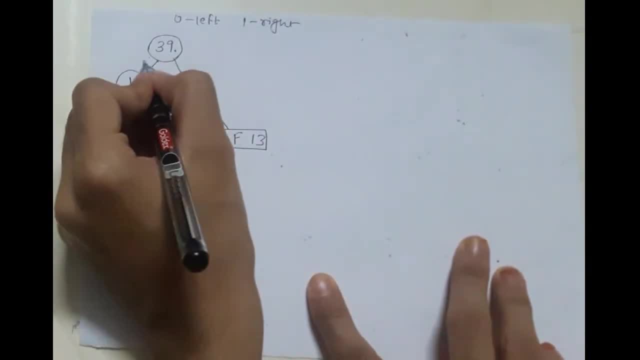 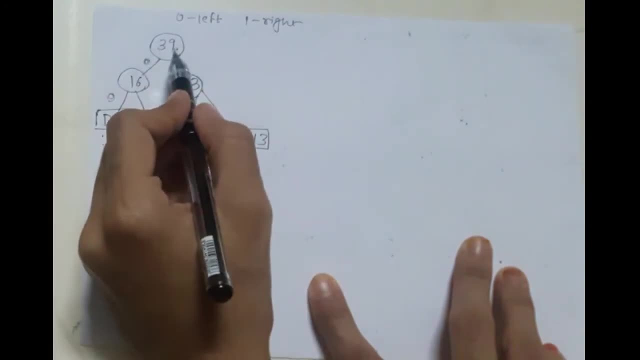 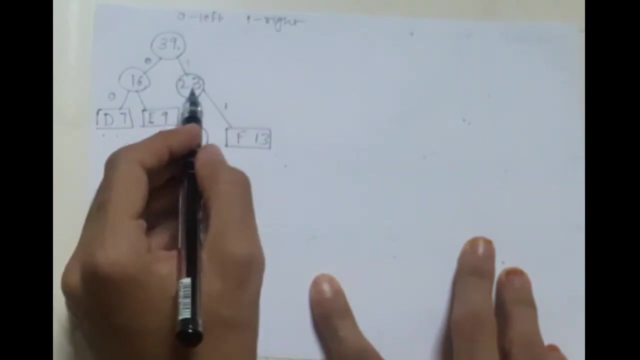 Okay, so left of 39 is 16.. So here 0 to its left is 7.. So 0 right of 39 is 23.. So here 1 right of 23 is 13.. So 1 left of 23 is 10.. 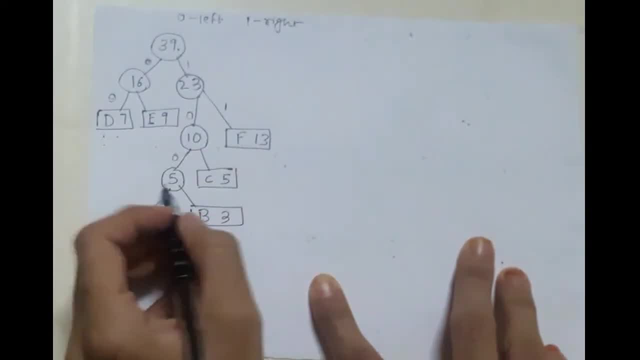 So 0 left of 10 is 5.. So 0 left of 5 is 2.. So 0 left of 10 is 5.. So 0. so it is to the right, So it's 1.. 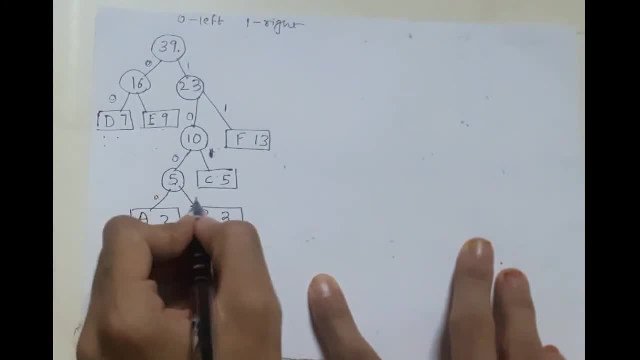 Okay, so right of 5 is 3. So here also 1.. Similarly, right of 16 is 9. So 1.. So in this way we will assign 0 and 1 to this half-man tree. 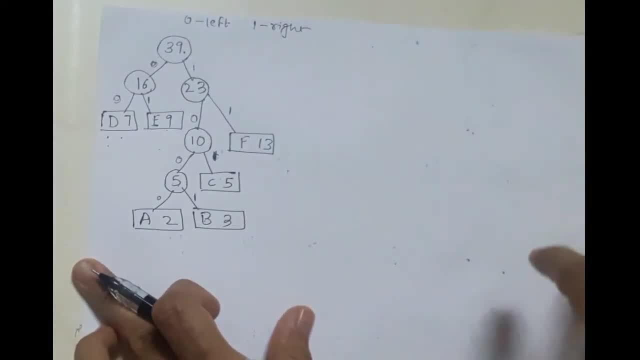 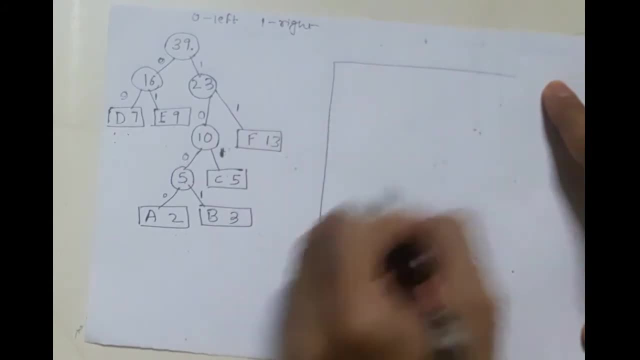 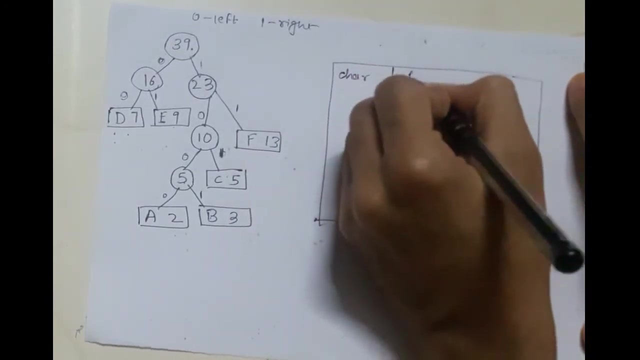 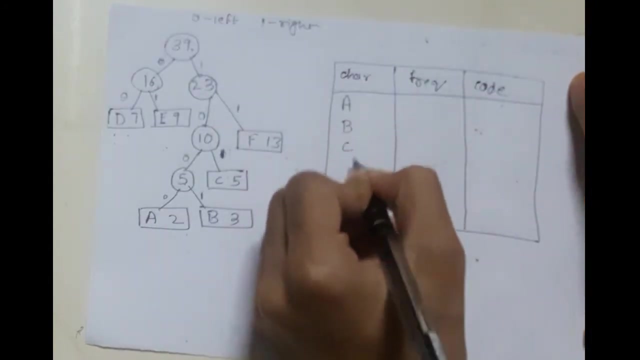 And after assigning- And this what we will do, We will find the half-man coding for each character Right. So I will create one table here. I will write code and everything in that table. Character Frequency and code. Frequency of A is 2.. 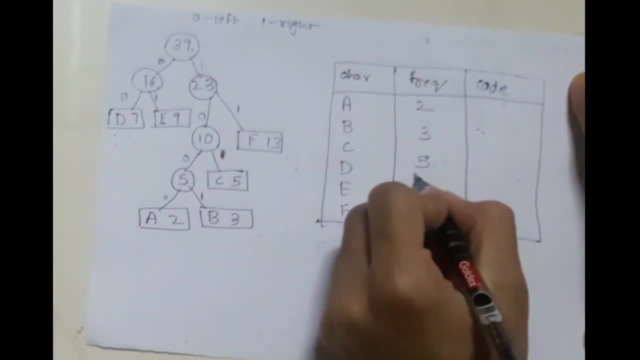 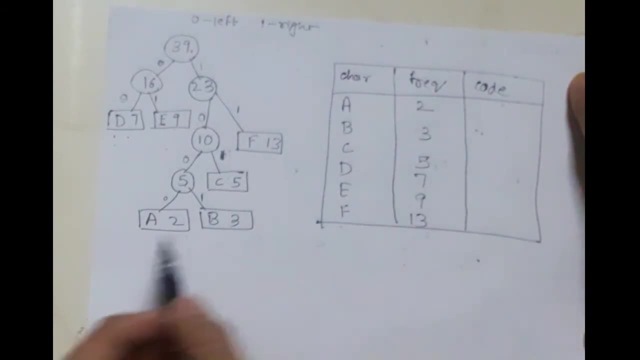 B is 3,, C is 5,, D is 7,, E is 9,, F is 13.. Now we will find the code for each characters. So for finding code of A, Here there is A. So what we will do. 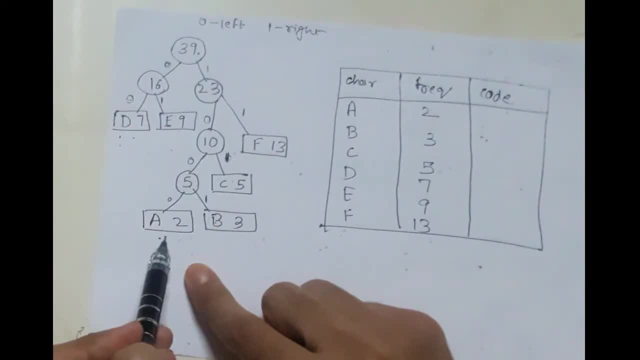 We will traverse this tree. So we will traverse it from root to the leaf. That is A. So each, you can see each character is the leaf node. So we will traverse the tree from root to the leaf. So here we have to find a code for A. 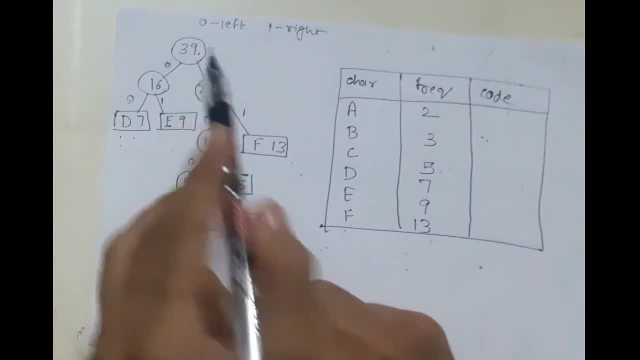 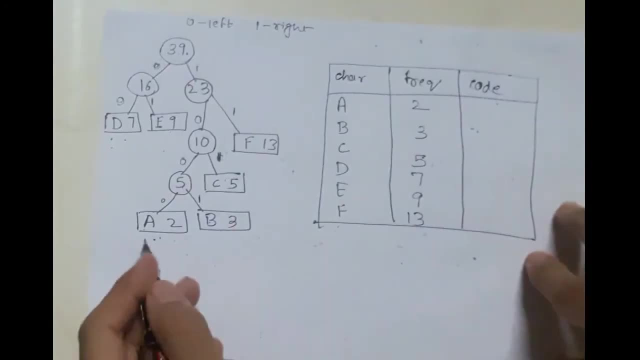 So we will traverse the tree from 39 to A. Okay, So what we can see Here, there is 1, 0, 0, 0.. Right, So the code for A is 1, 0, 0, 0.. 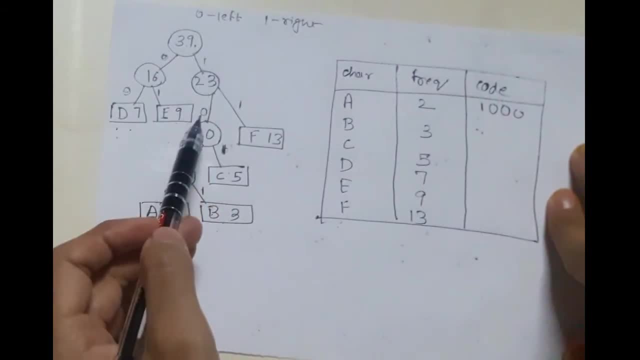 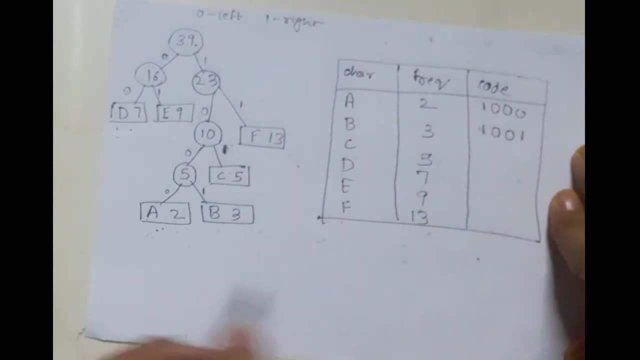 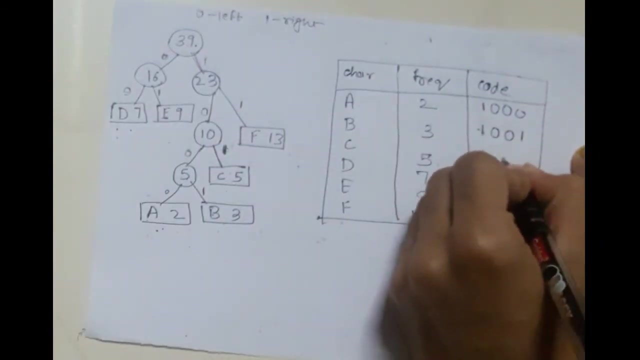 Similarly B. Here it is 1, 0, 0, 1.. Okay, So 1, 0, 0, 1.. Then C: 1, 0, 1. 1. 0, 0, 1.. 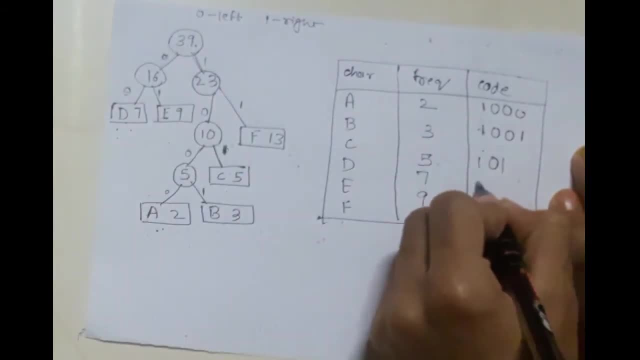 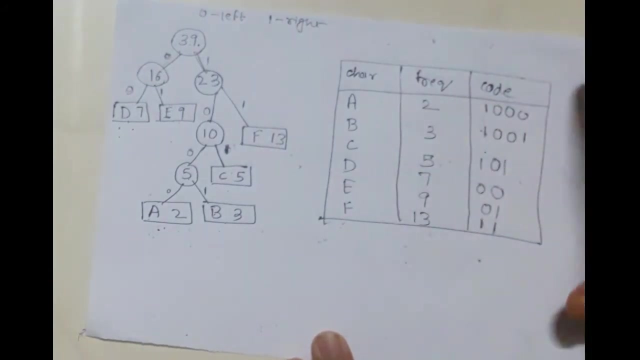 D- 0, 0.. E- 0, 1.. F- 1, 1.. Okay, So these are the codes for the respective characters. Right Now, by looking at this table, we can make two observations. 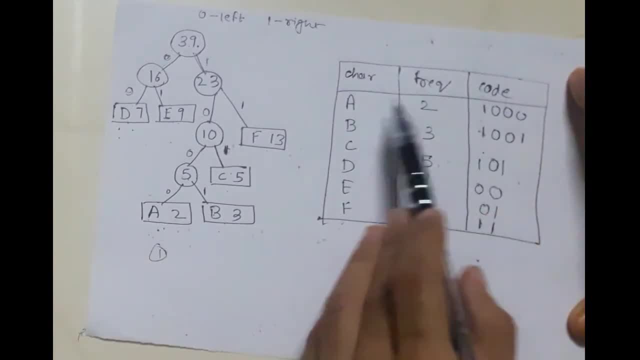 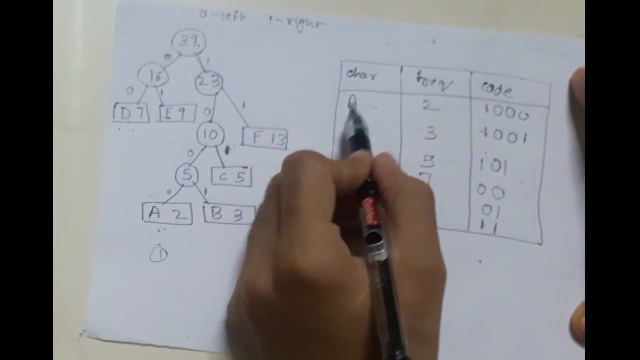 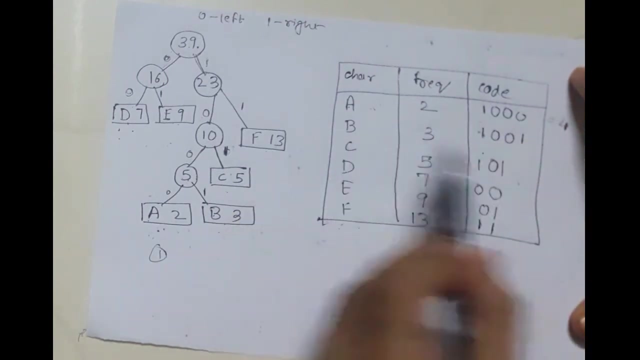 The first observation is that, see, every character is having different codes. Right variable code, see a, has code 1 0, 0, which is which is having length 4. right c is having code 1 0, 1 and its length is 3. e is having code 0, 1 and its length is 2. f is having code 1, 1, its length is 2. 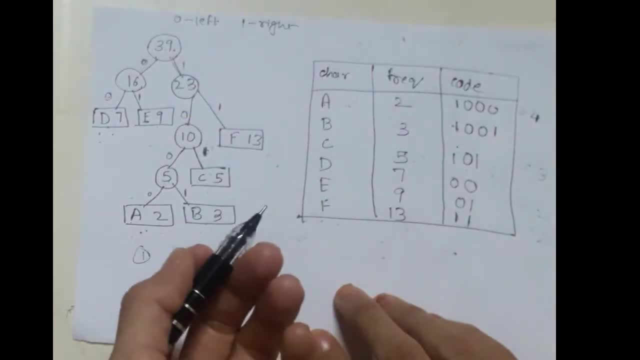 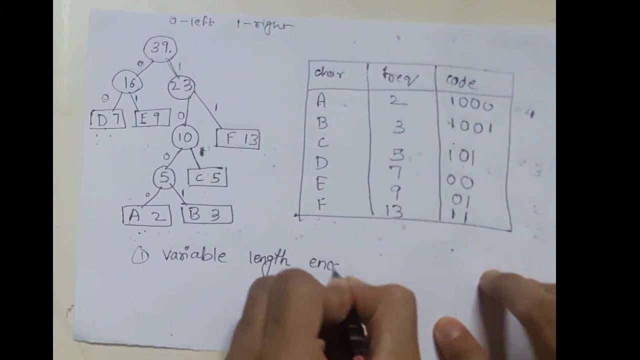 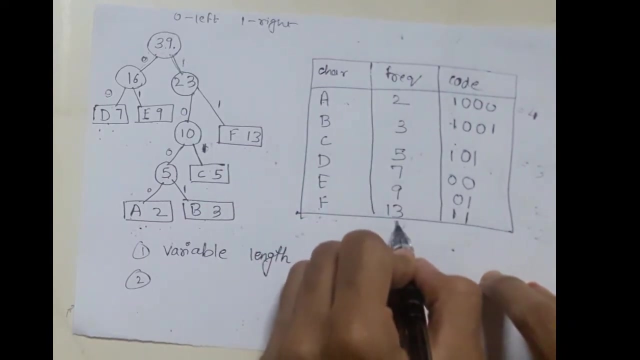 so, like this, every character is having different code. that is variable code and the length are also variable. so it we can say it is variable length encoding, variable length encoding right now. the second observation which you can make is that, see, f is having frequency 13, which is the highest among 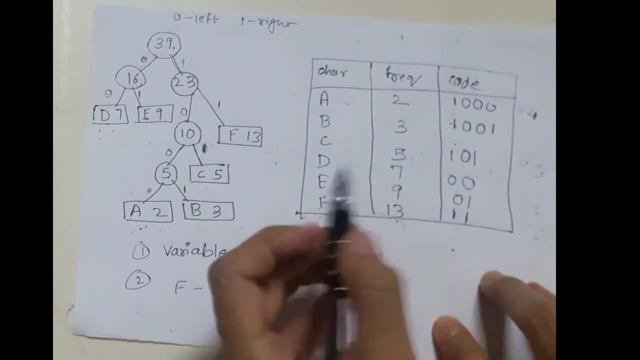 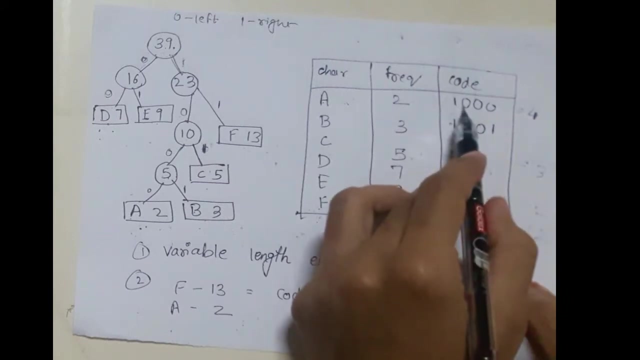 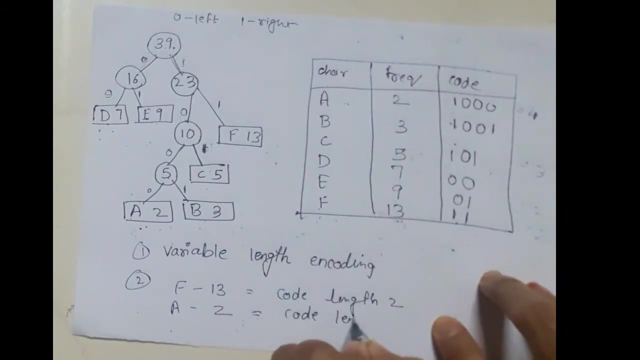 all. f is having frequency 13, which is highest among all, and its code is 1, 1, which is of length 2. code length 2 right. a has frequency 2 and its code is 1, 0, 0, 0, which is of length 4. code length 4 right. so from: 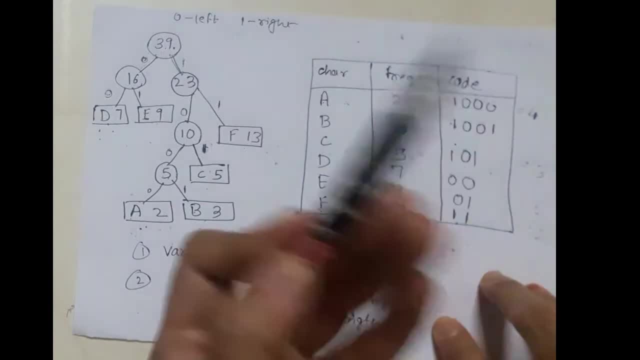 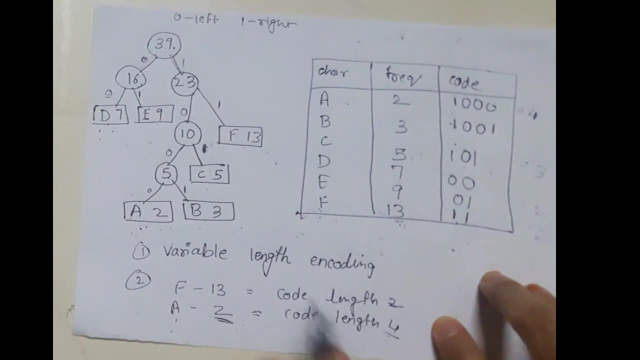 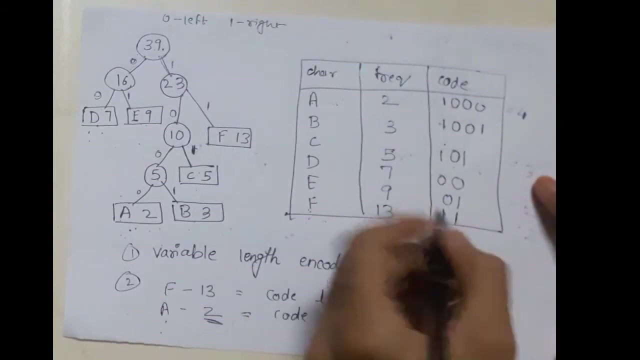 this you can conclude that the character which have highest frequency has code length small and the character which has least frequency has code length big. so these are the two observations which we we can make from this table. and also Huffman coding follows the technique of prefix code, prefix code. so now 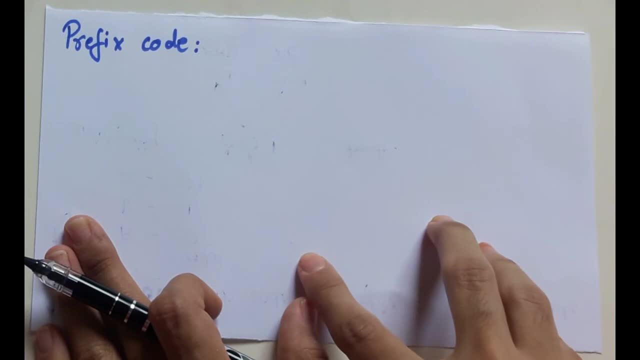 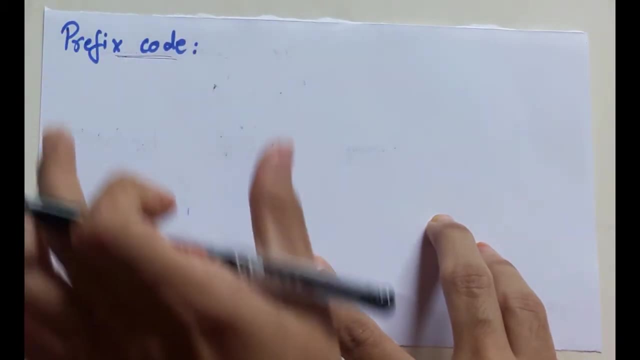 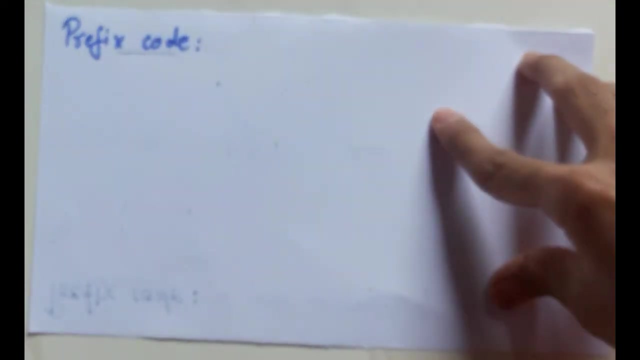 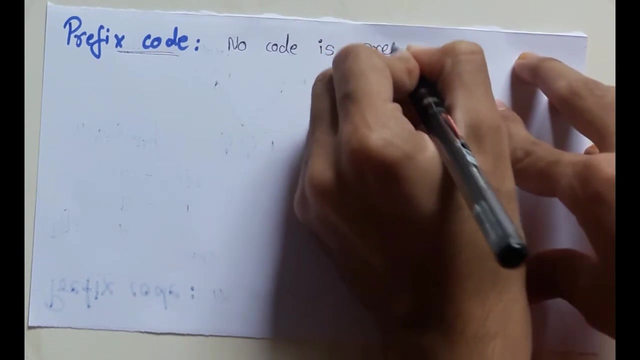 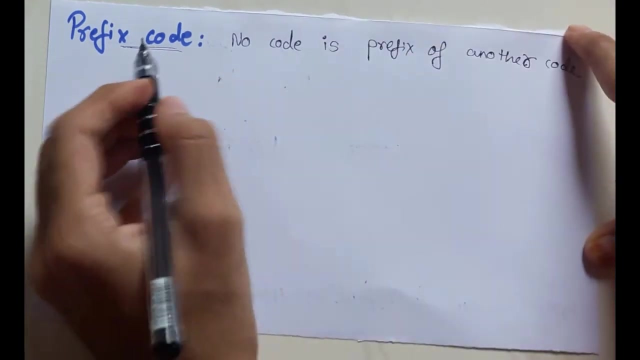 let us see what is this prefix code. okay, now let us understand what is this prefix code, and Huffman coding ensures this prefix code. also, it is called as prefix rule. okay, and what does prefix code says? or what does prefix rule says: no code is prefix of another code. what does this rule says: no code is prefix of another code. now let us. 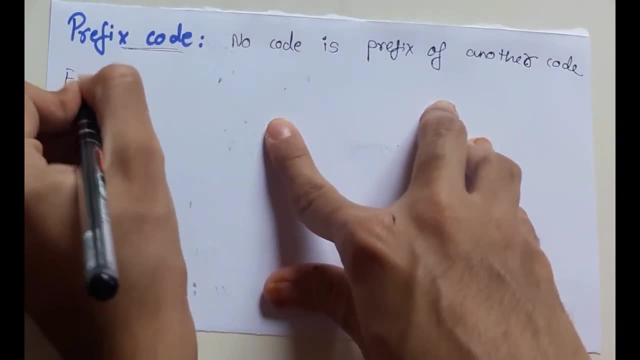 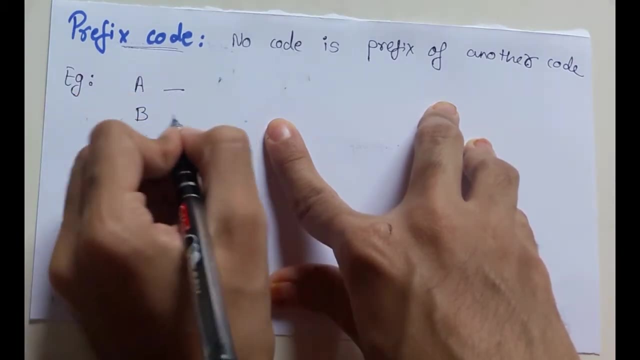 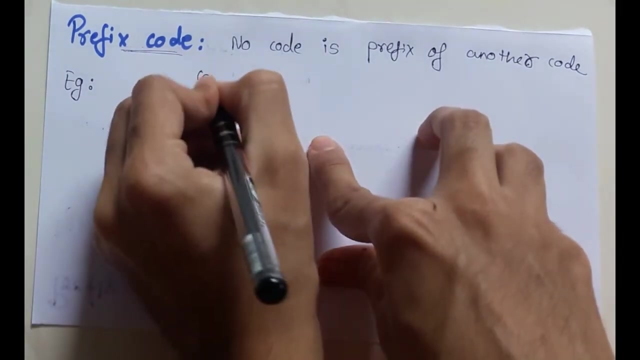 understand this with the help of an example, very simple example I'll take. see, suppose we have three characters, a, B and C, and their codes are 0, 1, 0, 1. okay, these are the characters and these are its codes. okay, and now one message is sent from: 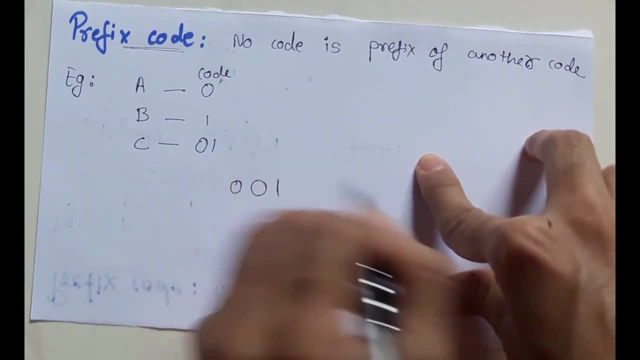 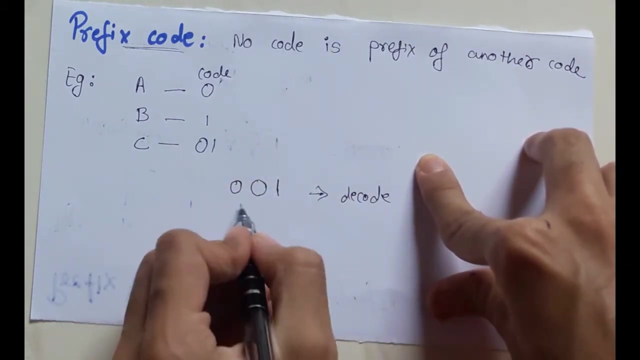 sender to receiver and that message is 001. it is encoded, okay, and what the receiver will do? the receiver will decode this message. when this message will be received by the receiver, the receiver will decode this message. now there will be ambiguity while decoding this message, because this single message will be decoded into two ways. see how. the first way: 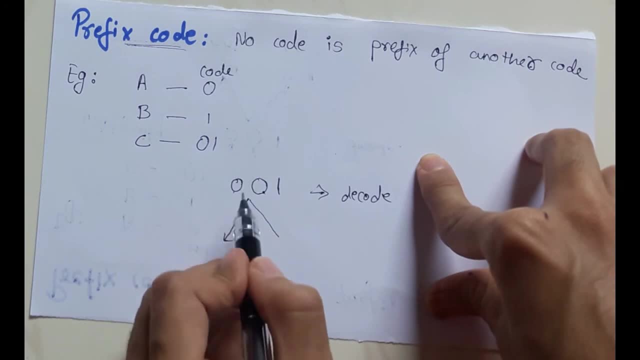 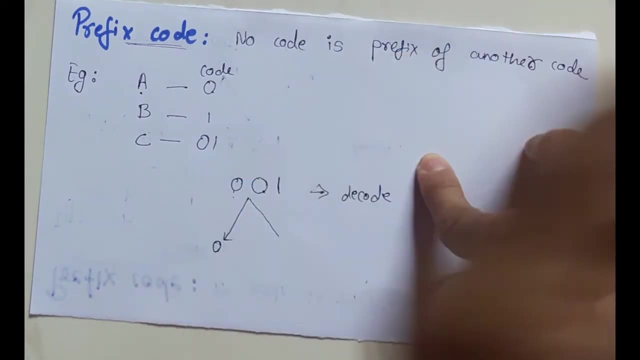 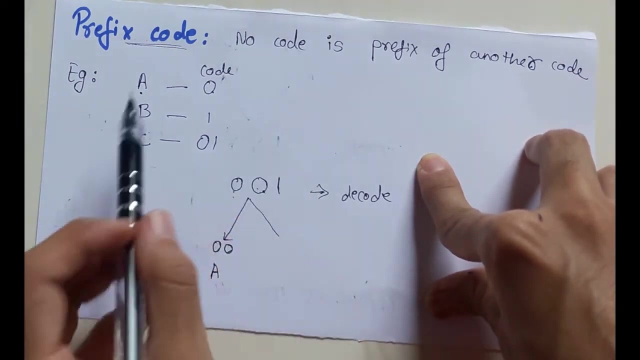 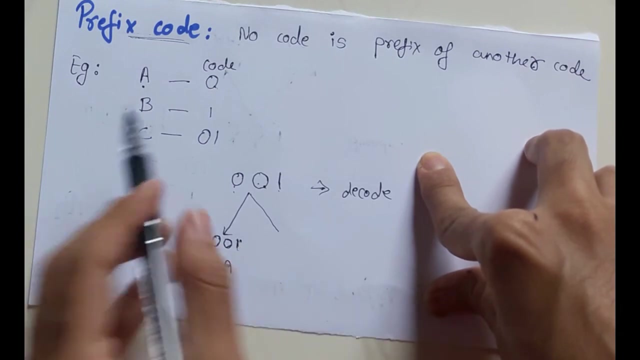 is now. see the first. there is 0. first bit is 0, the character with code 0 is A. so for first bit, what does the receiver will decode A? next bit: again 0, the character with code 0 is A, and then third one is 1 and the character with code 1 is B. so this is one solution. now another solution. 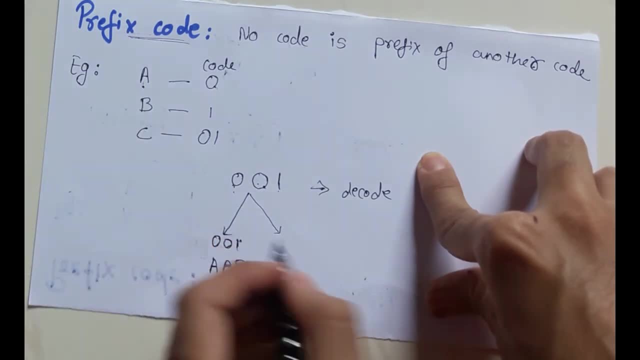 first bit 0, code of A is 0, so 0, then together 01. the character with code 01 is C, so here there will be C, C, right? so this is another way. now you can see that the sender is sending only one message and receiver is decoding into two ways. so this is nothing but ambiguity. right now, how?